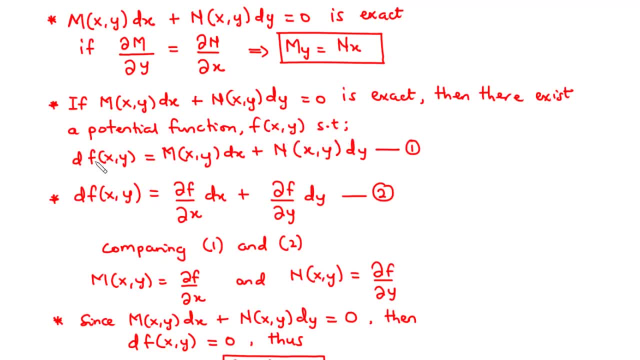 is a function of x and then y, such that the derivative of the function is equal to m of x- y, dx, plus n of x, y, dy. Now let's call this equation one. Now again, the derivative of the function f of x- y is said to be nothing but the partial derivative of the. 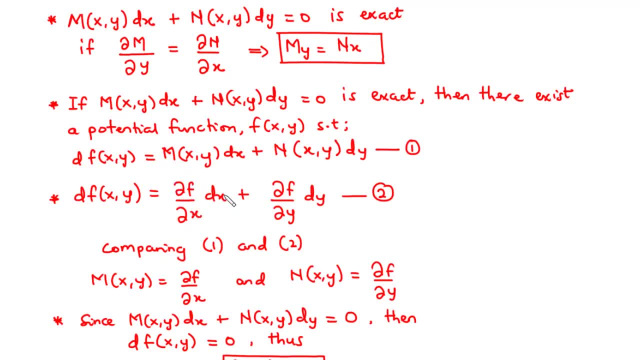 function f with respect to x times dx, plus the partial derivative of the function f with respect to y times dy, and we call that equation two. Now notice that the partial derivative of the function with respect to x and the partial derivative of the function with respect to y, 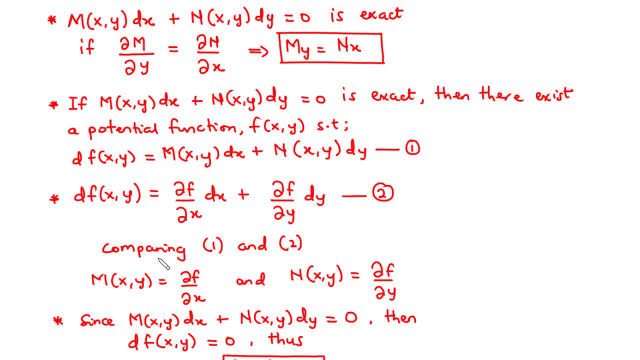 are all functions of x and y. Now, comparing the two equations here, you realize that the function m of x- y is equal to the partial derivative of f with respect to x, and then the function n of x- y is also equal to the partial derivative of f with respect to y. 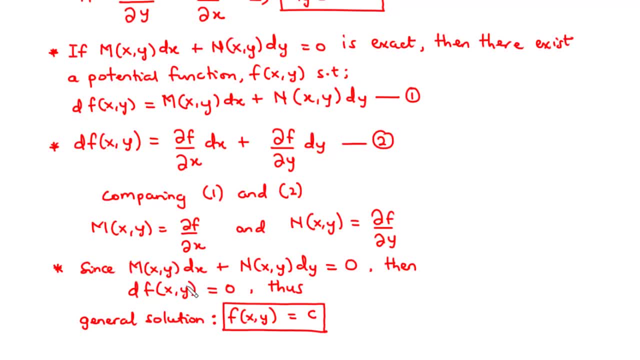 Now, since the exact differential equation, which is m of x- y, dx plus n of x- y- dy, equals zero, then what this primarily means is that the derivative of the potential function f of x- y is also equal to zero, and thus the general solution of any exact differential equation. 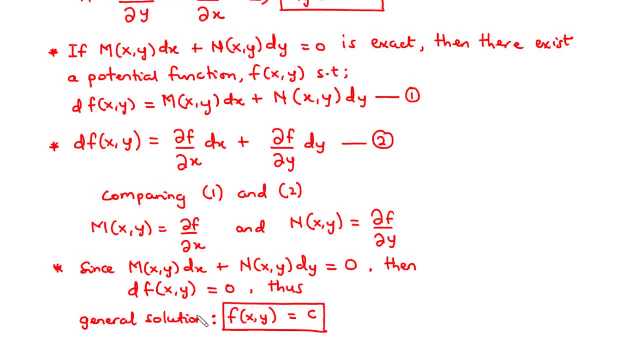 is of the form f of x. y equals c, where c is a constant. Now, basically, in today's video, what we are going to do is, given a differential equation, we are going to test the function of x and y. So let's start with the equation. 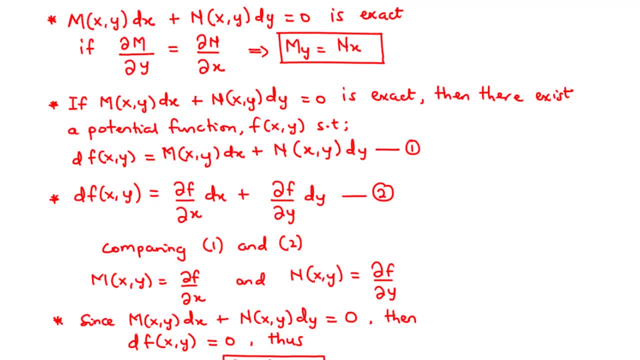 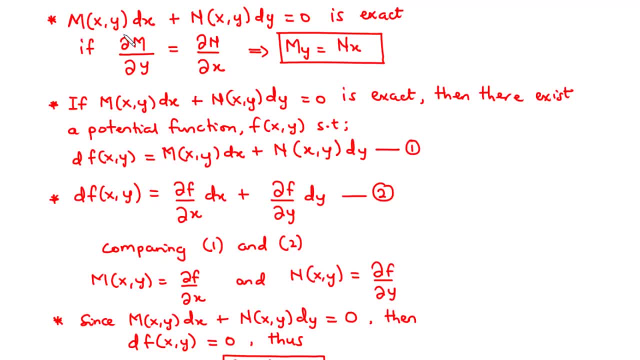 Notice that a differential equation of the form m of x, y, dx plus n of x, y, dy equals zero is said to be exact if the partial derivative of m with respect to y is equal to the partial derivative of n with respect to x. So now let's move on to the next section, where we are going to take. 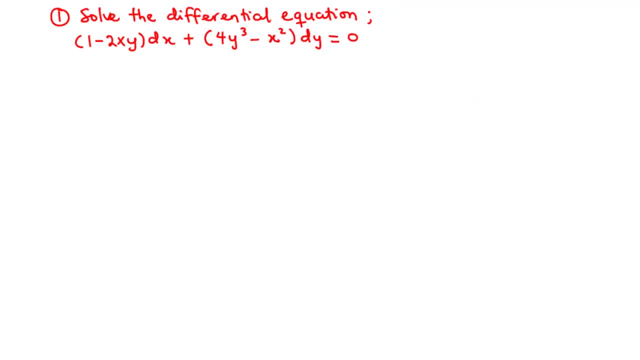 a couple of examples. So in our first example we are going to solve the differential equation 1 minus 2 x y dx plus 4 y cube minus x, squared dy equals zero. So the first thing we need to do is to test for exactness. 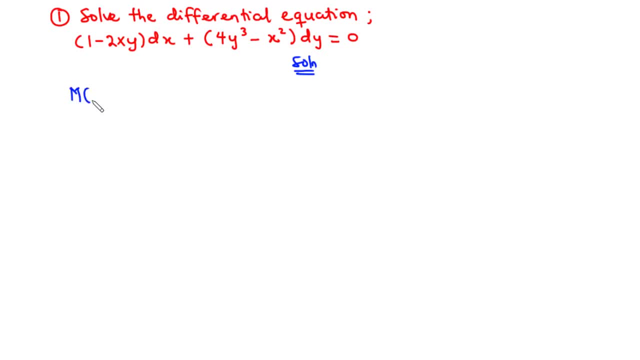 Now, in the previous section we said that a differential equation of the form m of x, y, dx plus n of x, y, dy equals zero is said to be exact if the partial derivative of m with respect to y is equal to the partial derivative of n with respect to x. 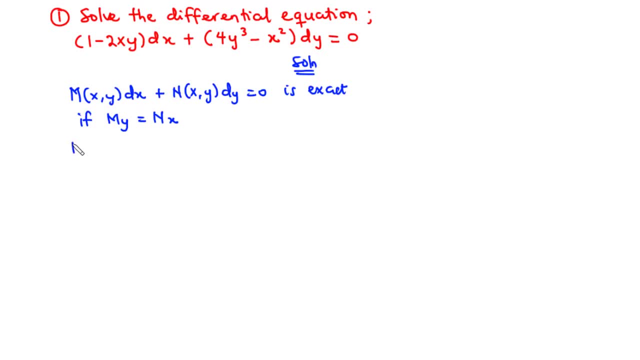 Now, comparing these two equations, you realize that we have the function m of x- y to be equal to 1 minus 2 x- y, and then the function n of x- y also to be 4 y cube minus x squared. Now the next thing we are going to do is to find the partial derivative of m. 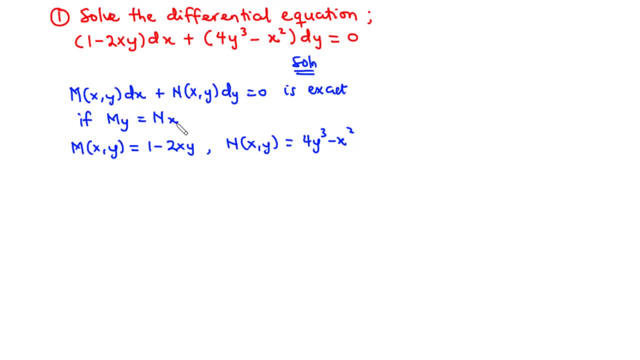 with respect to y and then the partial derivative of n with respect to x and see whether they are equal. So we have m, y and that is equal to Now to find the partial derivative of m with respect to y. what we are going to do is we are going to perform differentiation on y and then we treat x or any. 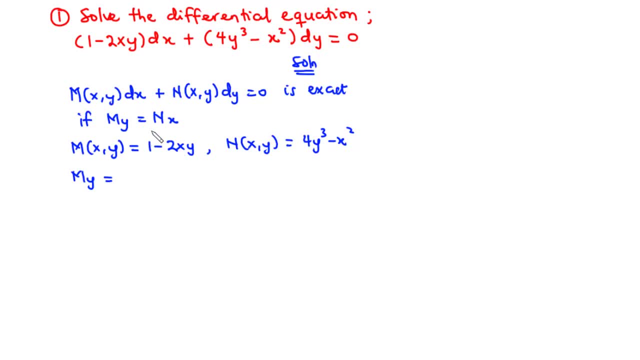 other value to be a constant. Now, when you differentiate 1 with respect to y, you are going to have 0 and then you have minus. You are going to treat 2x as a constant, so you are going to perform differentiation on y. Now, derivative of y with respect to y is 1.. So 1 times 2x is 2x. 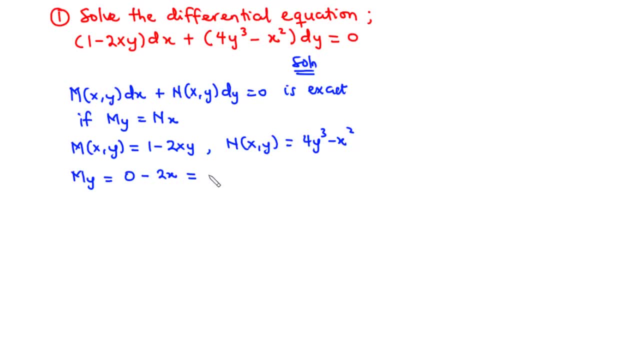 So you have 2x and then you simplify this as negative 2x. So that is the partial derivative of m with respect to y. Now let's move on to nx: partial derivative of n with respect to x. So the same way you are going to perform differentiation on. 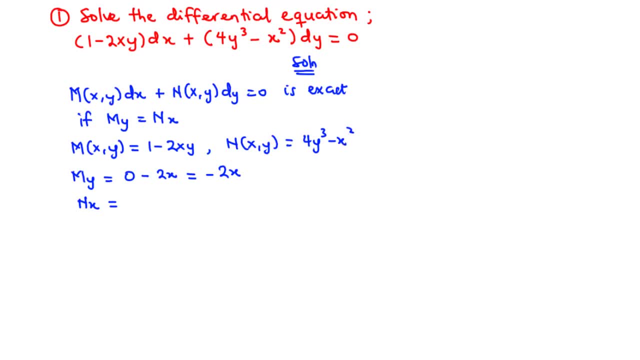 x, and then you treat y and any other value as a constant. So when you differentiate 4y cube with respect to x, you are going to have 2x, So you have 2x, and then you simplify this as negative 2x. 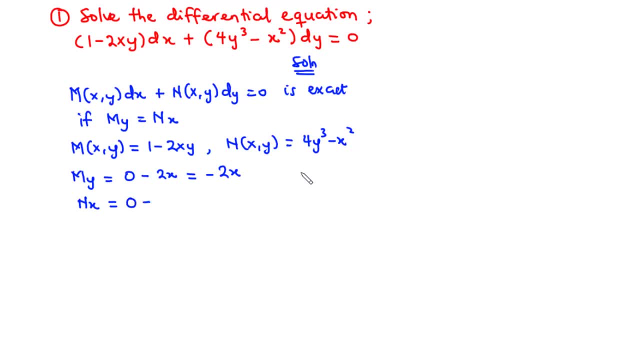 So you have 0 minus. when you differentiate x square with respect to x, then you are going to have 2x. Therefore, we have nx to be equal to negative 2x. Now, since the partial derivative of m with respect to y is equal to the partial derivative of n with respect to x, it follows that: 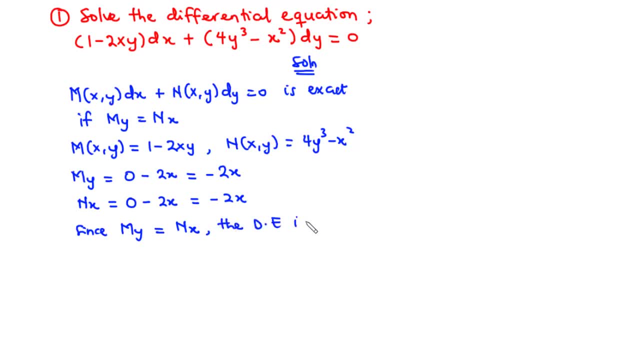 the differential equation given is exact. The differential equation given is exact. So the next thing we are going to do is to perform integration on the function m of xy and then n of xy. Now we are going to integrate m of xy with respect to x, and then we integrate the function n of xy. 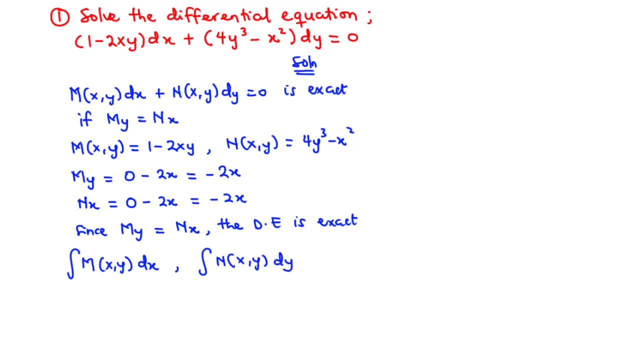 with respect to y, and then we merge the two functions. So that is what we are going to do. So for the integral of m of xy- dx that is equal to now. we have m of xy to be 1 minus 2xy, So that is equal to the integral of 1 minus 2xy dx. Now let's try to solve further. 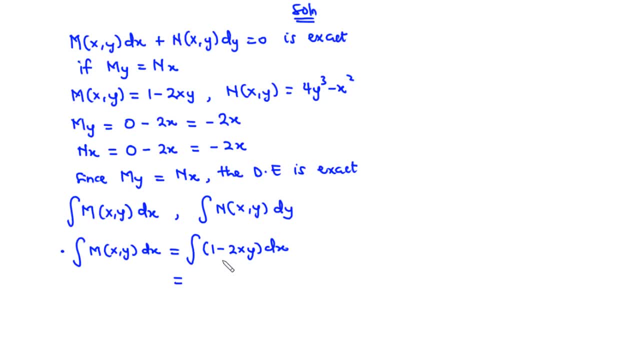 So this time we are going to perform integration on x and then we treat y as a constant. So when you integrate 1 with respect to x, you have x and then minus. We are going to perform integration on x, So you maintain 2y. So this is 2y. Now, when you integrate x with respect to x, 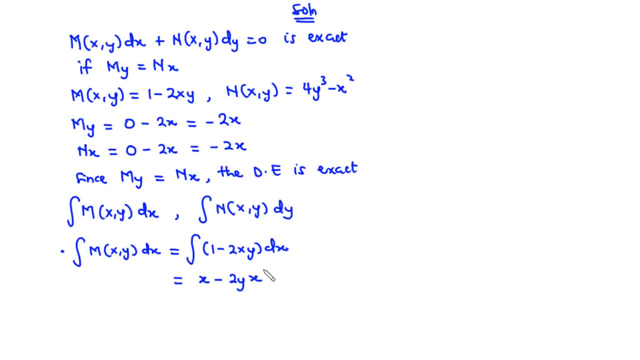 then you have x, and then you increase the exponent by 1.. So 1 plus 1 becomes 2, and then you divide by the total exponent, which is 2.. Now, in this case we are going to neglect the arbitrary constant of integration. So we simplify this so that we have: x minus 2 cancels out 2.. 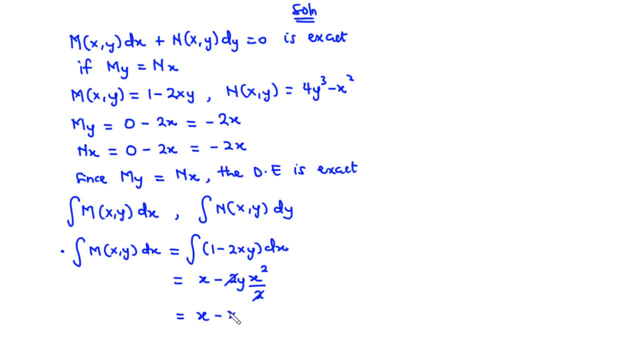 We are left with x square y, So minus x square y. So that is the integral of the function m of xy with respect to x. Now let's move on to the integral of n of xy with respect to y, So we have the integral of. 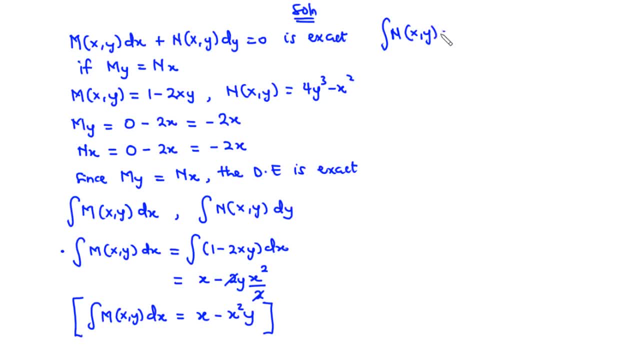 n of xy with respect to y equals. we have integral of. that becomes 4y cubed minus x square dy. So let's solve this together. Now we are going to perform integration on y, And so here we have 4y cubed. 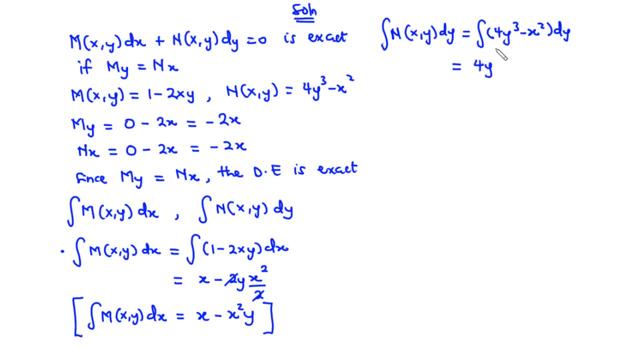 So we perform integration, that becomes 4y. We increase the exponent by 1.. 4 divided by the total exponent minus, here we have x square times 1.. So when we integrate 1 to y then we are going to have y. So that becomes x square times y. 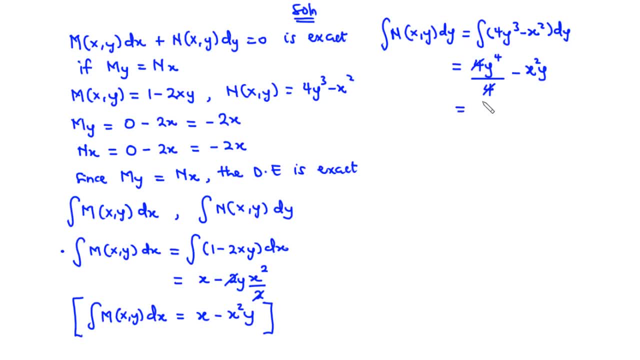 Now 4 cancels out 4.. We are left with y exponent: 4 minus x square times y. Notice that at this point also, we are going to ignore the arbitrary constant of integration. So we have the integral of n, of xy, dy to be y to the power: 4 minus x square times y. 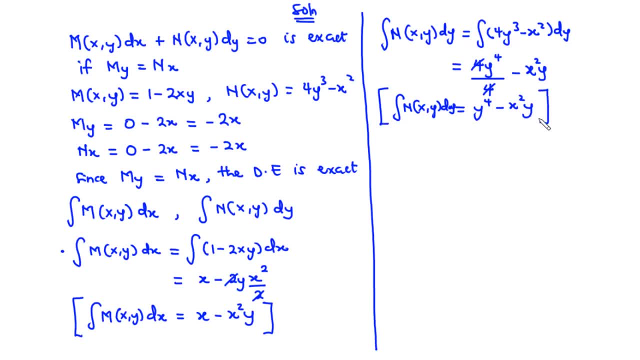 Now the next thing we are going to do is to merge the two functions, So we have the function f of xy to be equal to now. at this point we are going to write each term only once. we are going to merge the two functions and then we write each term. 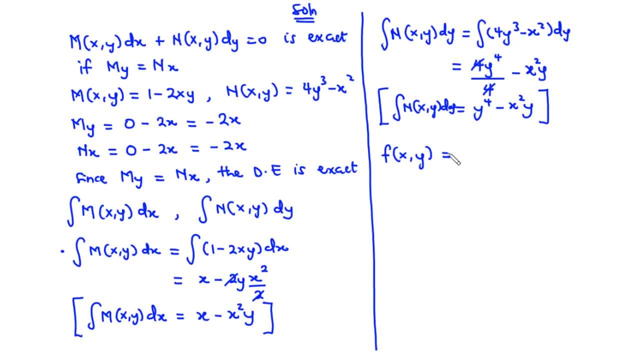 only once. So we start with this function, we have x and then minus x square y, and then we move on to that function. we have plus y to the power 4 and then notice that here we have negative x square times y, which has already been written here. 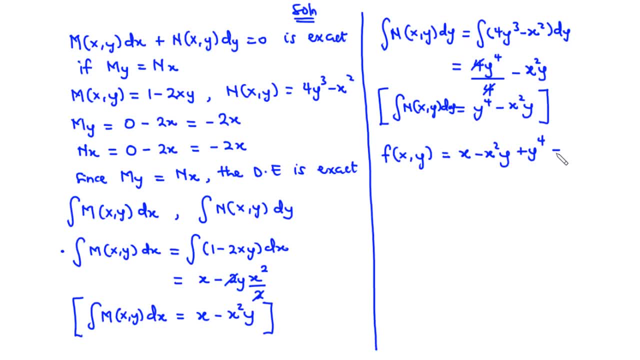 And so we ignore that. The additional one, And then this is equal to c. Now, since we are supposed to leave our answer in the form, since we are supposed to leave the answer in the form, f of xy equals c, then we say that we have our general solution to. 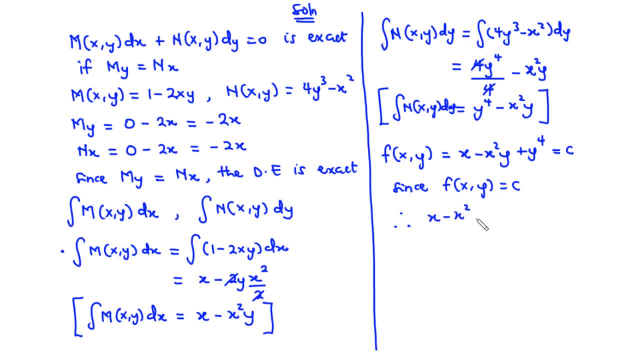 be x minus x, square y plus y to the power 4 equals c. So this happens to be The general solution to the differential equation. This is the general solution To the differential equation. So basically, this is how to solve an exact differential equation. 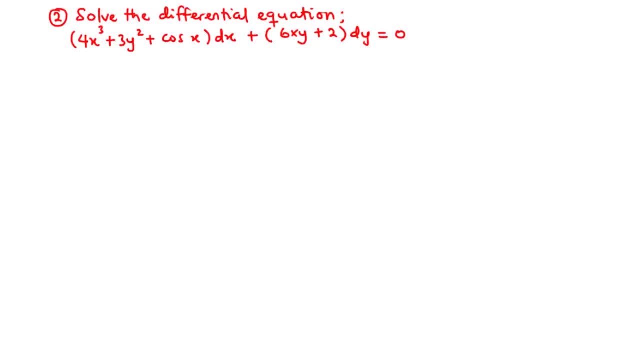 Now let's move on to the second example. So in our second example we are going to solve the differential equation For xq plus 3y, square plus cos x, dx plus 6xy plus 2, dy equals x. So here we are going to solve this differential equation. 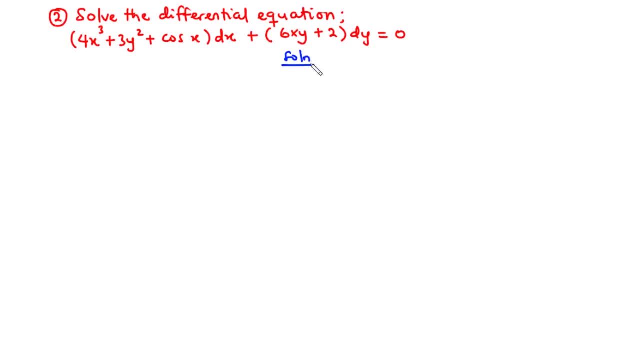 So in this differential equation we have m of xy equals 4x cube plus 3y square plus cos x, and then we have n of xy, also to be equal to 6xy plus 2.. Now for the differential equation given to be exact, then it means that the partial derivative of m with respect to y must be equal. 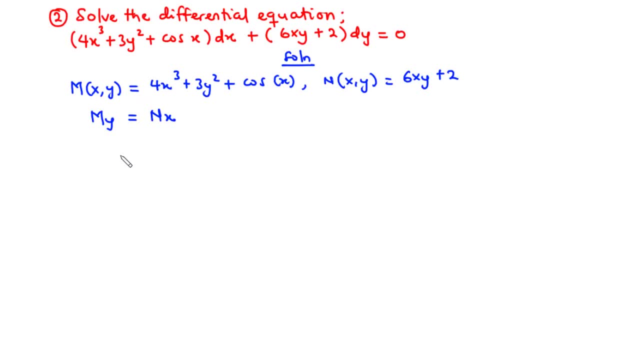 to the partial derivative of n with respect to x. So let's find the partial derivative of x. So we are going to perform differentiation on y, and then we consider any value or any other variable- let's say x in this case, to be a constant. So when we differentiate, 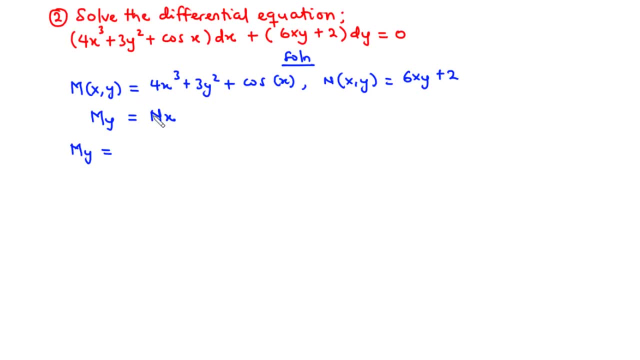 4x cube with respect to y, then we have 0. plus when we differentiate 3y square with respect to y, we have these two, the exponent multiplying 3, so that we have 6, and then y, and then we reduce the exponent by 1, so 2 minus 1 is. 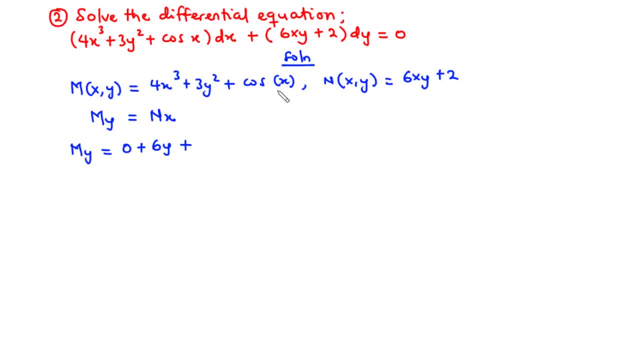 1, plus, when we differentiate cos x with respect to y, then that is 0. Therefore, we have my to be equal to 6y. Now to the partial derivative of n with respect to x. we are going to perform. 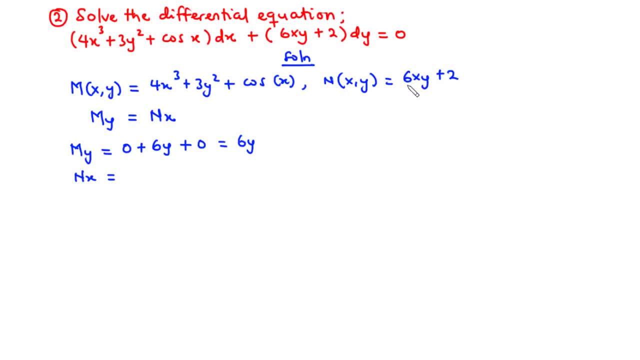 differentiation on x. So here we have 6xy. So 6xy, 6y becomes constant, so we have 6y. Now when you differentiate x with respect to x, then you have 1.. So 1 times 6y is still 6y. and then when you differentiate 2, which is: 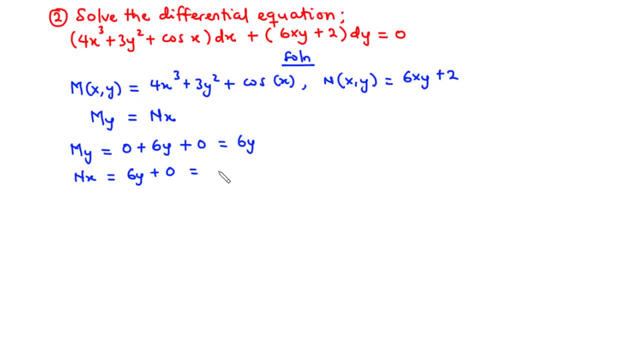 a constant. with respect to x, you have 0. So this is finally equal to 6y. Now, since the partial derivative of m with respect to y is equal to the partial derivative of n with respect to x, It follows that the differential equation given is exact. So the next thing we are: 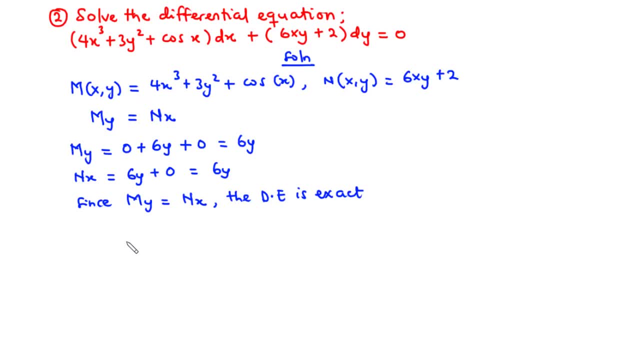 going to do is to perform integration on m and then n. So we are going to integrate m with respect to x. That is the first thing we are going to do. Later, we integrate n with respect to x, So we are going to integrate n with. 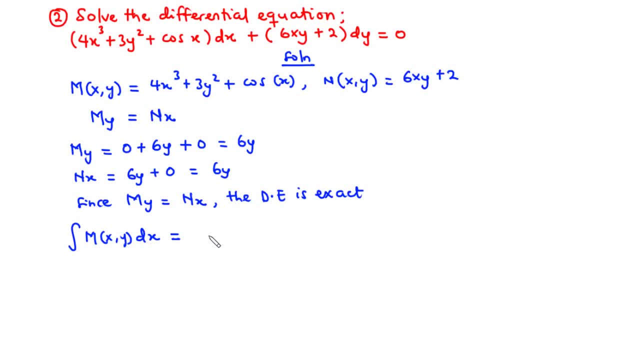 respect to y. so we have m of x y to be. that is, 4 x cube plus 3 y square plus cos x. so let's do this together. now we are going to perform integration on x, so we are going to integrate 4 x cube so that becomes 4 x. we increase the power by 1, so exponent 4 divided by the total. 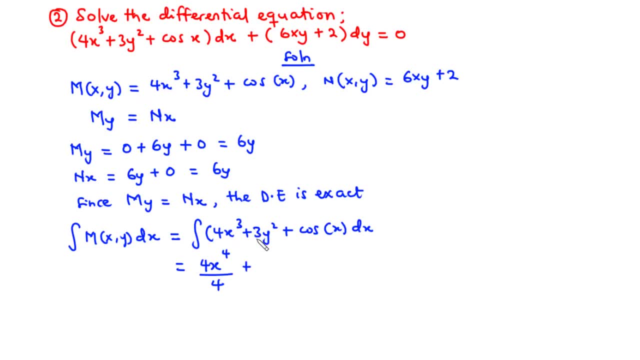 exponent, which is 4 plus. here we have 3 y square times 1. so if you want to integrate with respect to x, then we are going to have 3 y square x plus. when you integrate cos x with respect to x, then you have sin x. we are going to. 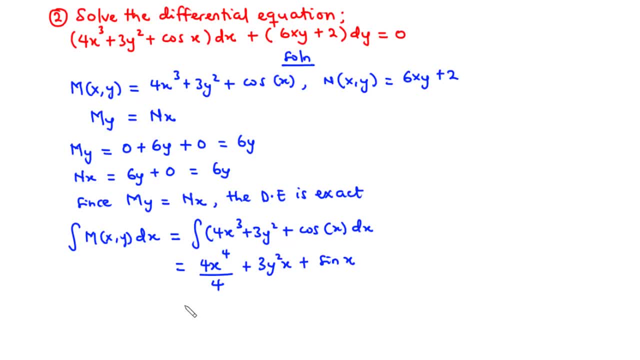 neglect the arbitrary constant of integration. so we simplify this: as 4 cancels out 4, we are left with x to the power, 4 plus 3, x, y square plus sin x, so that is the integral of m of x, y with respect to x. so now let's move on to the 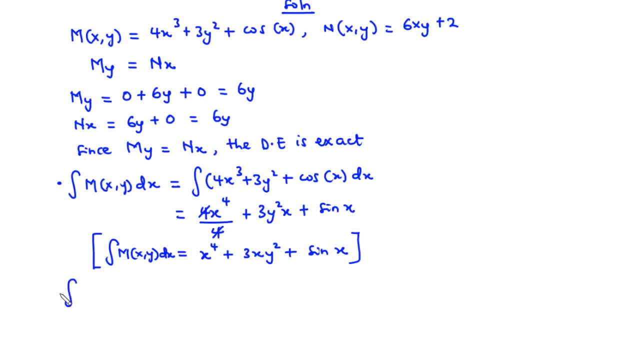 second one where we are going to perform integration on n of x- y with respect to y, so that is equal to. we have the integral of n of x- y, that is 6 x y plus 2 with respect to y. so we are going to perform: 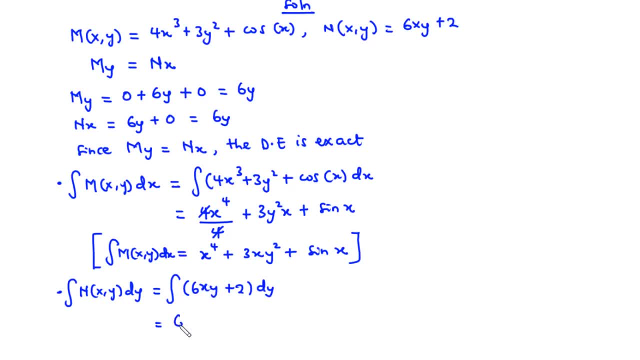 integration on y. so we have 6 x as constant and then we perform integration on y. so we are going to increase the exponent by 1. so we have y to the power, 2 divided by total exponent, which is 2, and then plus here is 2. so we integrate with respect to y and then we have 2 y. now we can simplify this. 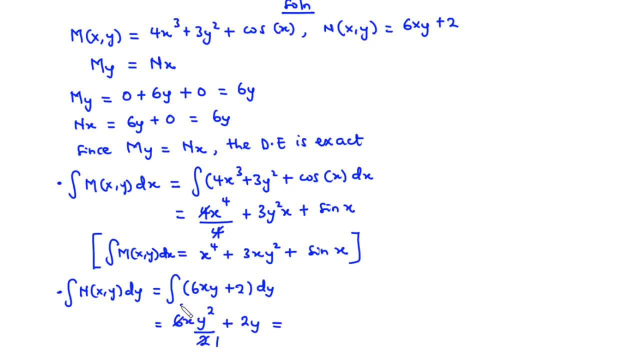 as 2 goes here once, 2 goes here 3 times, so that becomes 3 x y square x plus 2 y square x plus 2 y to the power of n of x i square plus 2 y. here also we neglect the arbitrary constant of. 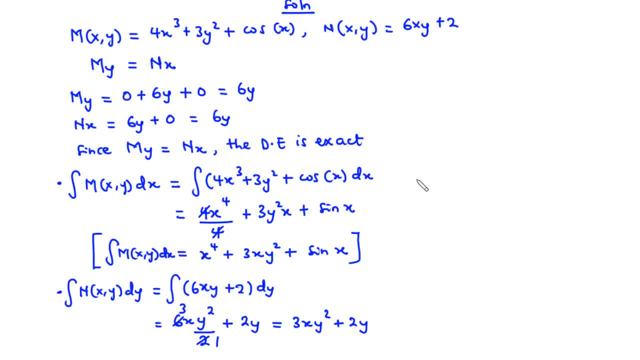 integration. now we are going to merge the two functions. ok, we are going to merge the two functions. we have this to be integral of n, of y, d, y, so we are going to merge the two functions. we are going to merge the two functions, so we are going to have 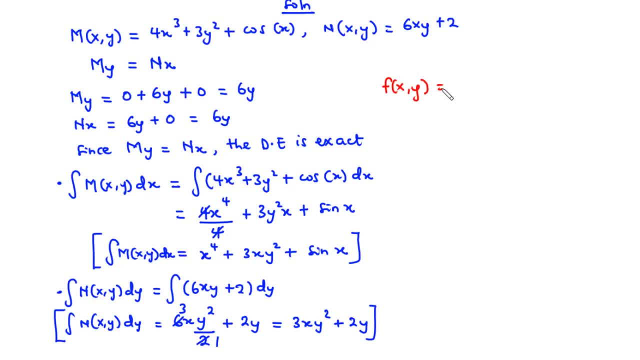 f to be equal to. as we merge, we are going to write each term only once. So first we have x to the power 4 plus 3xy square plus sine x, and then we move to the second function. we have 3xy square- repeating, so we ignore the additional one. and then here: 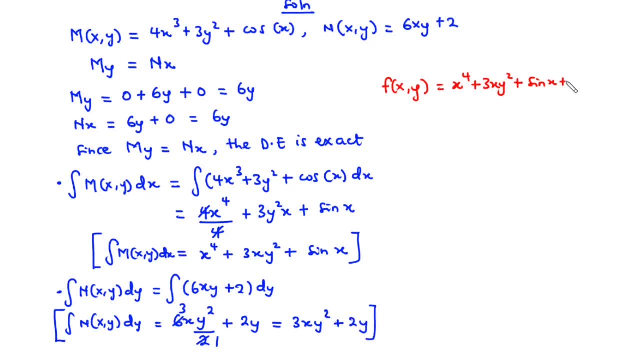 we have a new term: 2y, so plus 2y, and that is equal to c. Now, since we are supposed to leave our answer in the form f of xy equals c, where c is the constant. therefore, we say that the general solution to the given differential equation